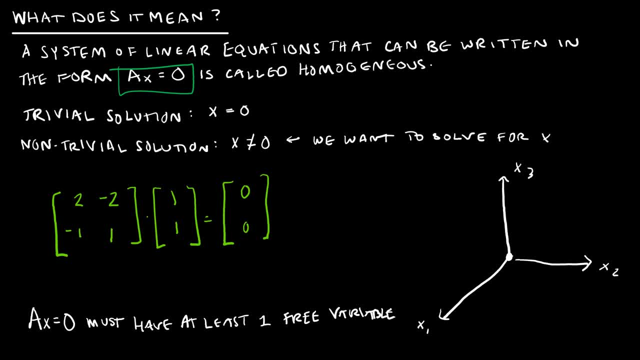 That is how I know it's called homogeneous. Now it makes sense that every homogeneous system would have a trivial solution of x equals 0. And what I mean by that is, if you'll recall, ax means I've got some matrix A. 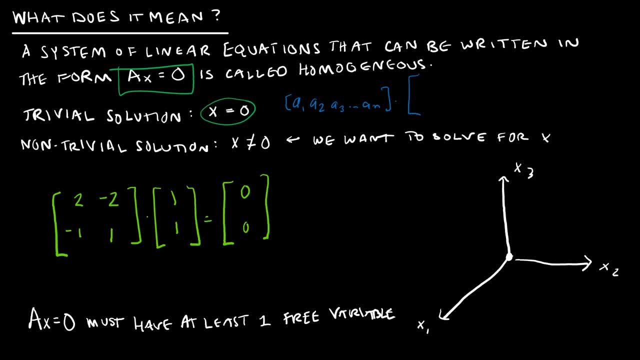 And it's multiplied by some vector x, And we're saying that that's equal to 0. So that's a homogeneous system. Why does it make sense? everything will have a trivial solution, Because if I replaced all of my x's with 0's, 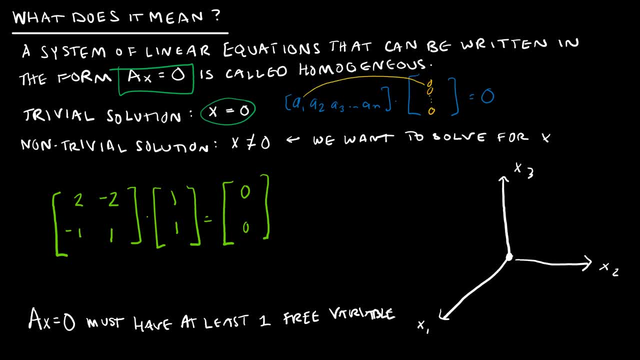 then it would make sense that everything would have a trivial solution And it would make perfect sense that A1 times 0 would be 0. Because, remember, 0 is just the 0 vector 0, 0 is all the 0's. 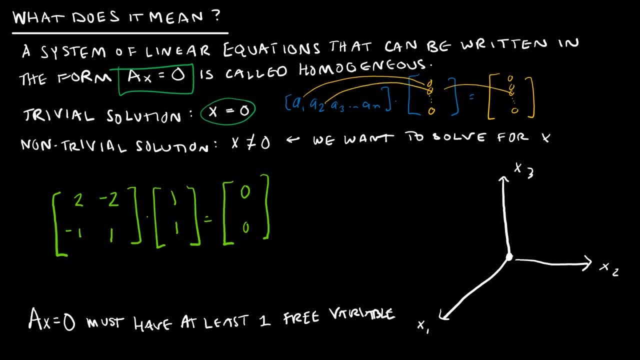 A1 times 0 is 0.. A2 times 0 is 0.. And we get the idea that it would make perfect sense that, no matter what I have here, if I have 0's in my vector, then my solution will be 0. 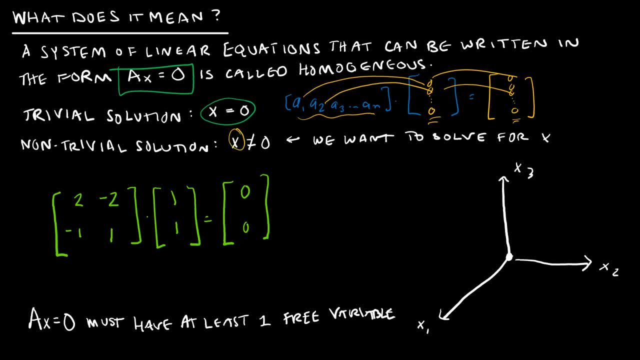 What we want to know is: is there some value for x- And we're talking about vector x, not just some variable? We want to know: is there some solution set that makes the matrix times the vector also equal to 0?? 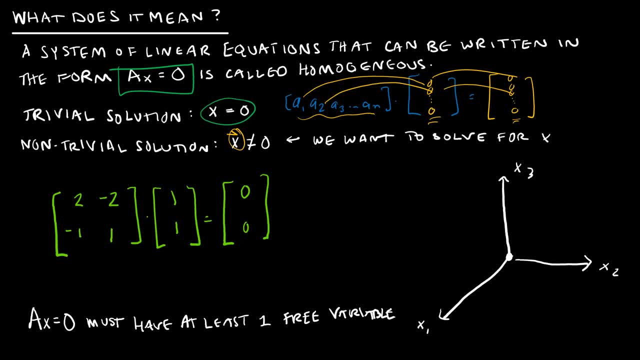 For instance, if I take a look at this matrix equation, if I took 2 times 1, plus negative 2 times 1,, that would be 0. And if I took negative 1 times 1, plus 1 times 1,. 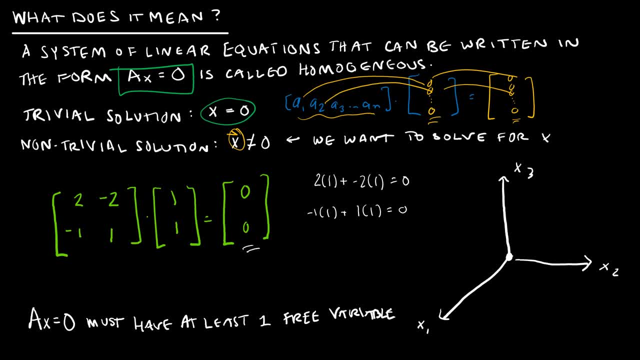 that would be 0.. And we can see that these are equal to 0, where this is A and this is x and this is 0, where x doesn't equal 0.. x itself doesn't equal 0, but when I multiply it by A, the solution is 0. 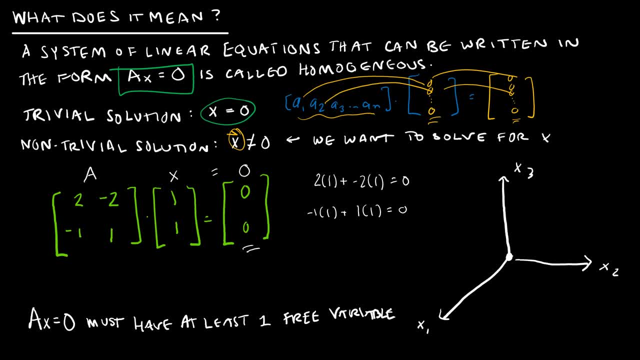 So that's an example of a non-trivial solution. Now, what would happen if, instead of 1,, I change these to 3s? Now what do I have? Well, 2 times 3 is 6.. Negative: 2 times 3 is negative, 6.. 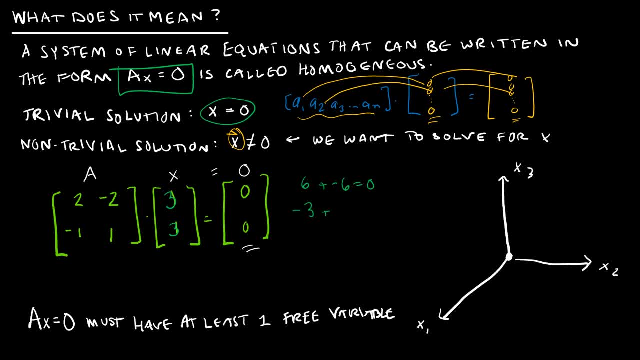 Yes, that still works. Negative 1 times 3 is negative 3.. 1 times 3 is 3.. And yes, that still works. So I could change my x vector to anything I wanted and still have a solution. 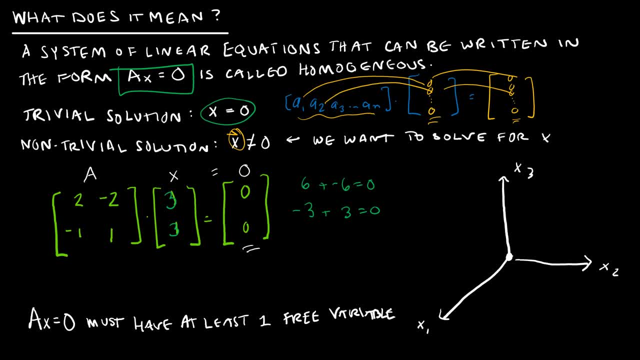 And so what that tells me is: I have a great many solutions, and whatever the solution is is dependent on some free variable. So that's how we know that we must have at least one free variable. What's that going to look like? 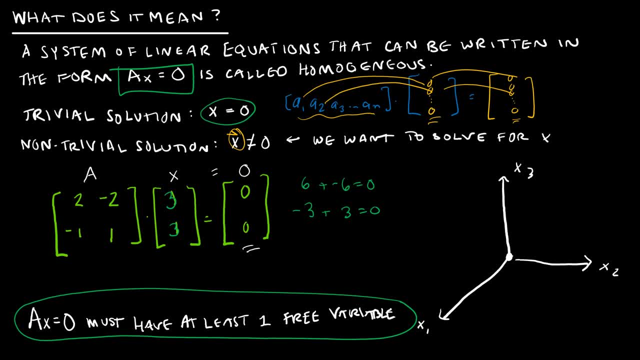 if I were going to graph that. Well, I would graph that if I had just one free variable, it would end up looking like a line that goes through the point, in this case, 0, 0, 0, because I've drawn this with. 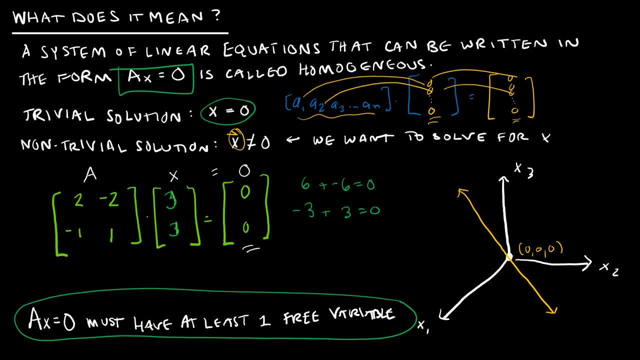 three dimensions or three variables, And if I just had one free variable, then it would look something like that. And the changes, or what makes the line, is I'm changing the value, of say, x1, and that is going to in turn. 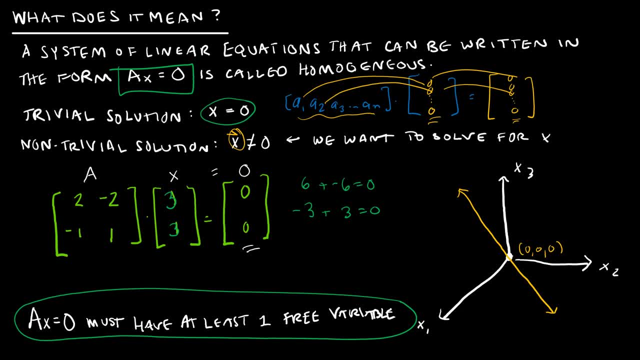 change the value of x2 and x3, because they were based on x1.. If I end up with two free variables- say x1 and x2 are both free, then x3 is going to vary based on 1, and so that will be what I change x1 and x2 to be. 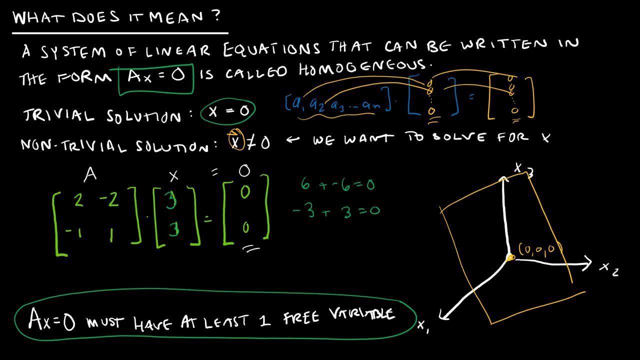 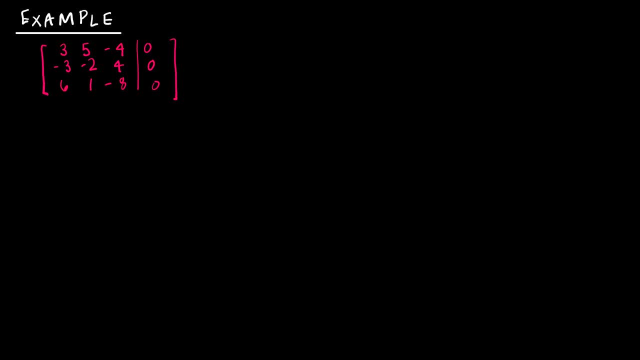 So it's going to end up looking more like a plane again, still crossing through that same point. So what I want to do is go through an example with you where we actually find what is our free variable and what are our other variables. 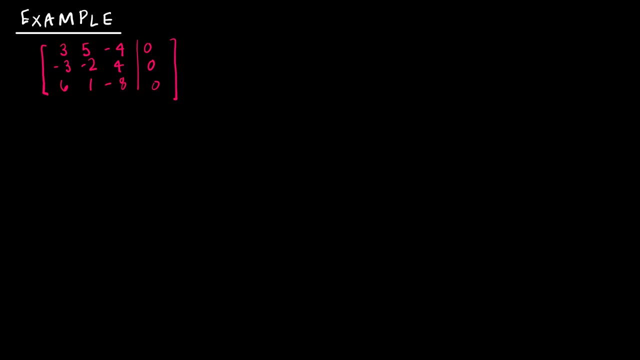 in relationship to that free variable. So here's an example: We have an augmented matrix- and I want to first write it form- where I have a on the left side and a is going to be an echelon matrix and zero obviously. 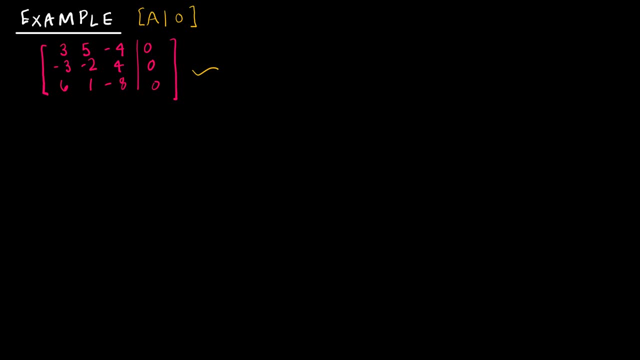 is the zero vector. So what I want to do is I essentially want to change these values all into zeros and to have my pivots at three and negative two. So let's take a look. Obviously, we should be really good at those row operations by now. Row one is going to remain the same, Row two I would. 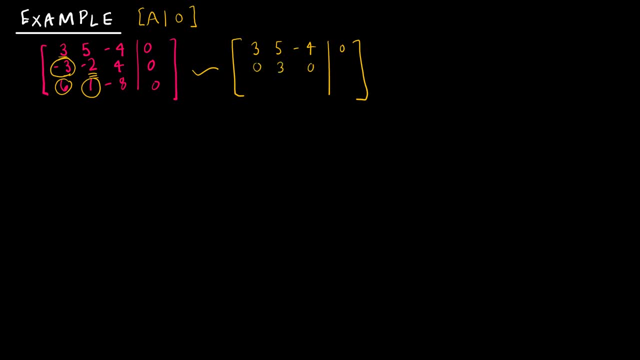 take row one plus row two to get zero, three, zero, zero. Row three: I would take negative two times row one plus row three and that would give me zero, negative nine, zero, zero. Now, from here, I want to, and I really want this guy, of course, to be my pivot, which means below that, I still would like to have a zero, because at first, 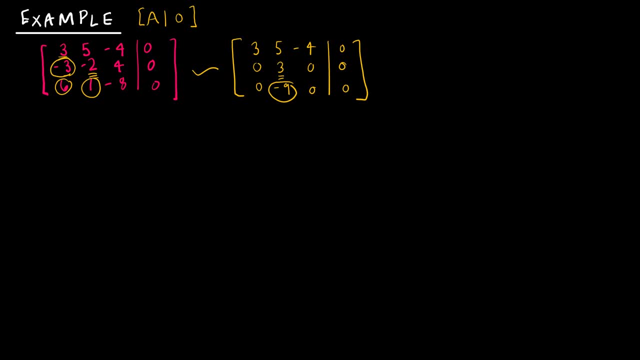 I just want to look at echelon form. So what's going to happen now is not a darn thing. on row one, row two: not a darn thing, row three: I'm adding three times row two to row three. so zero, zero, zero, zero. So at this point, before I get to the end of the row, I'm going to be able to. 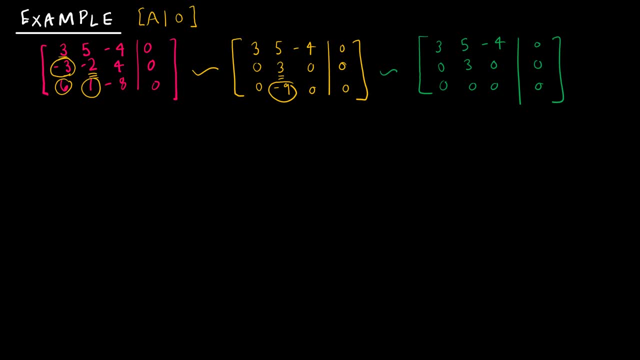 continue. So, before we continue, what does this tell me? This tells me again: keep in mind, this is the x ones, x twos, x threes. I've got a pivot in x one and a pivot in x two, and obviously no pivot in x three, which tells me that x three is free. Now, what I want to do from here is continue my 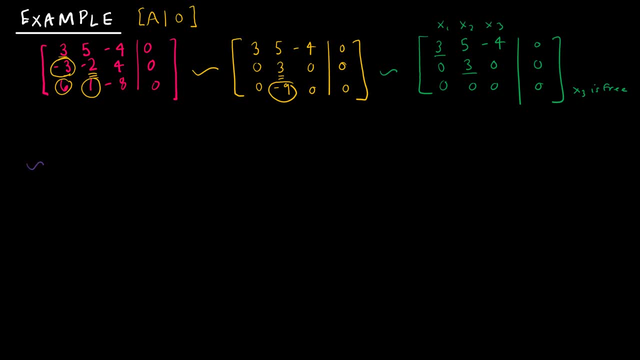 row operations so that I have, instead of threes, where my pivots occur. I would like those to be ones. So, for instance, I have a pivot in x one and a pivot in x two and obviously no pivot in x three. So what we do now is: I will take the x and the Dedate in x, please, So this one has zero. 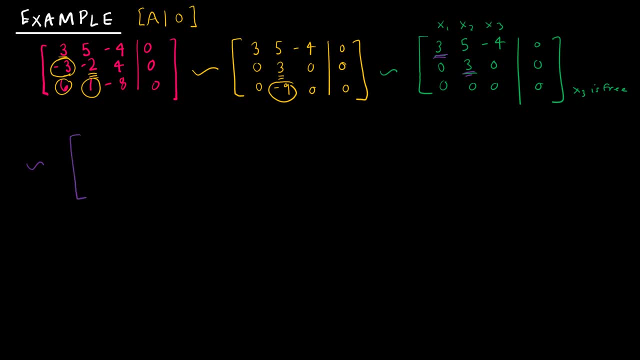 and we wouldn't also be able to keep anything but a perfect extreme set in here, Since I might take a third of row one to get one, 5 thirds negative, 4 th귀rds zero, and a third times row two to get zero, one, zero, zero, and row three would remain unchanged. and then I would take: 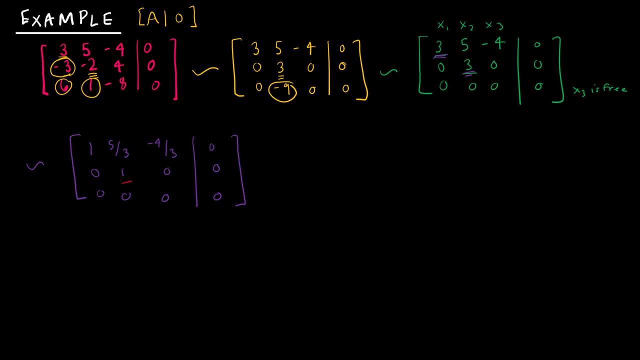 it one step further, because if I have a one here then this guy must be a zero. so I'm going to take negative Pfe with challenge row three times row four, So the x, thos, x, twos, x, threes are equal to zero. and then Heraus, five thirds negative E. 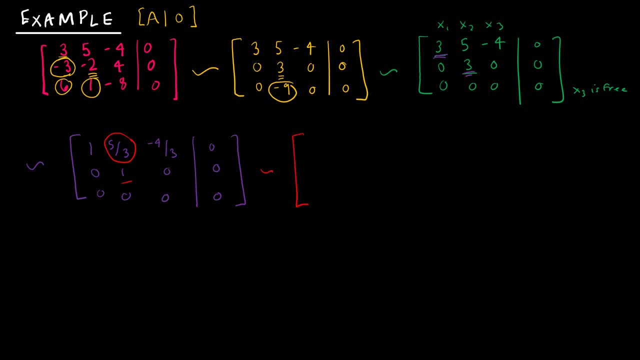 2 and add it to row 1.. So now I have 1, 0, negative 4 thirds: 0, 0,, 1, 0, 0, and 0, 0, 0, 0.. 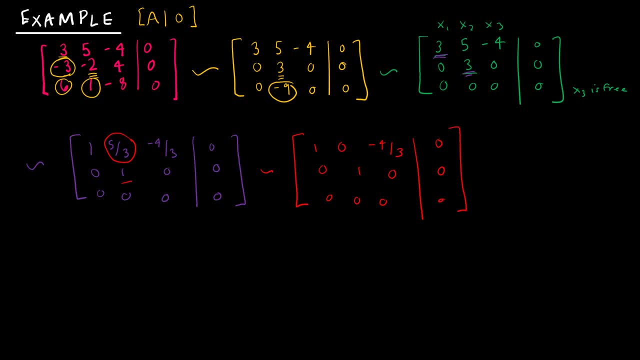 So in our last video, this is kind of where we ended and we said: great, but here's my solution set, because this, of course, is x1, x2, x3. So instead of writing x1 minus 4 thirds x3 equals 0, we said: x1 is equal to 4 thirds x3. And x2 is equal to 0. 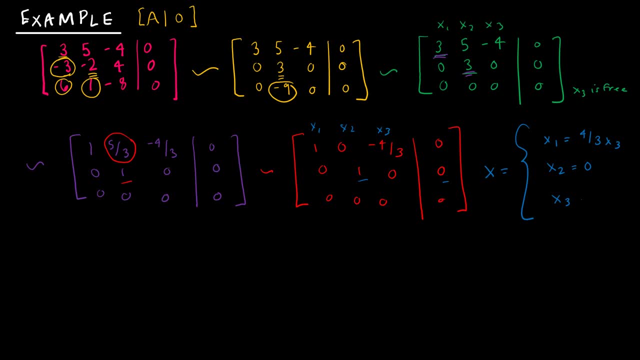 And x3, we already said, is free. So that's kind of where we stopped on the last video, and I want to continue Now just a little bit further, because that's what we do in mathematics: is we just always keep? 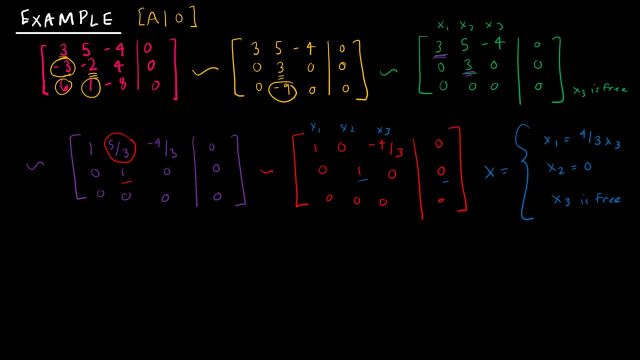 pushing, and, pushing, and pushing. So what am I going to do from here? Well, let's say I wanted to write this instead as a vector, because that's what I want- is vector x to be x1,, x2, x3.. 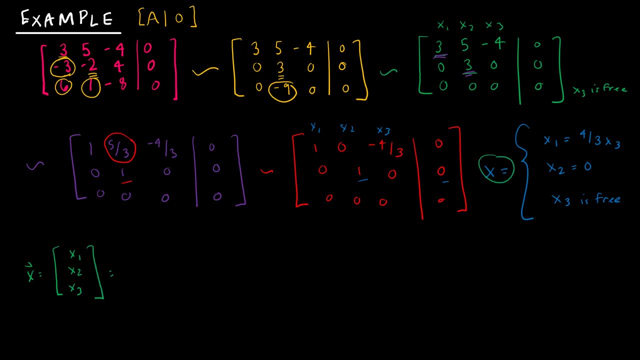 So vector x then, based on this guy, is that x1 can be written as 4 thirds x3, x2 can be written as 0, and x3 is free, so I'm just going to write x3.. And what I notice now? 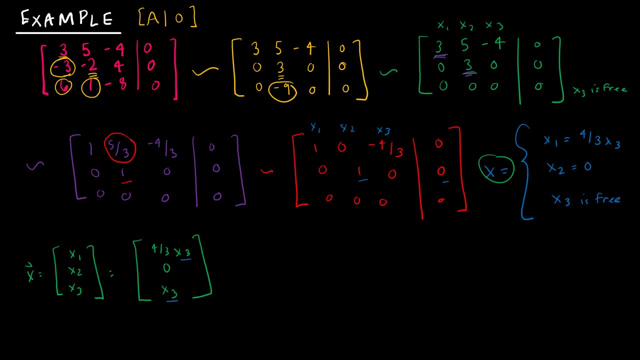 is that my terms have an x3, so I'm actually going to take x3 out of it and write this as 4 thirds 0, 1.. So what I have is that my solution is now some constant x3, which I don't know what x3 is, but some constant x3 times vector v. 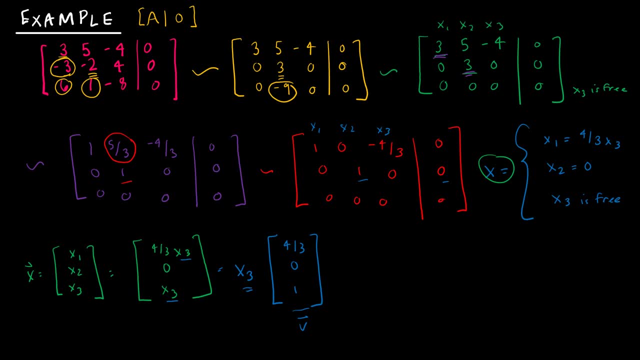 So this brings us to parametric vector form, and parametric vector equation essentially says that I can write x as some constant times some vector, And so I'm going to write x as some constant times some vector. So essentially what I'm saying is that x3 is t, because I want to write it as t v. 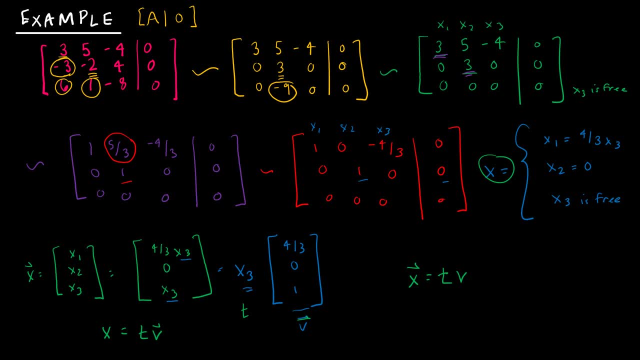 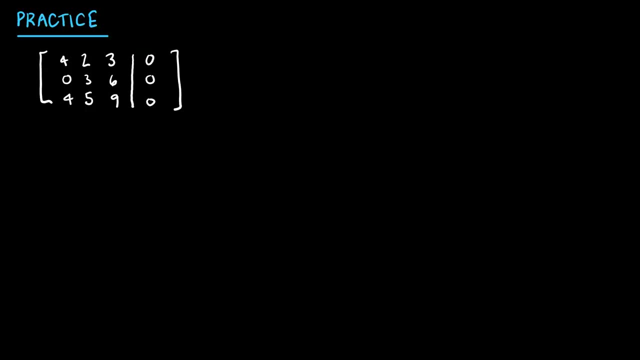 And that's what I have is. I have now written this as in the parametric vector equation form. Here's one for you to try, before we make things a bit more complicated. So this should be pretty straightforward, like our last example. So if you would press pause, try to do what we did on our 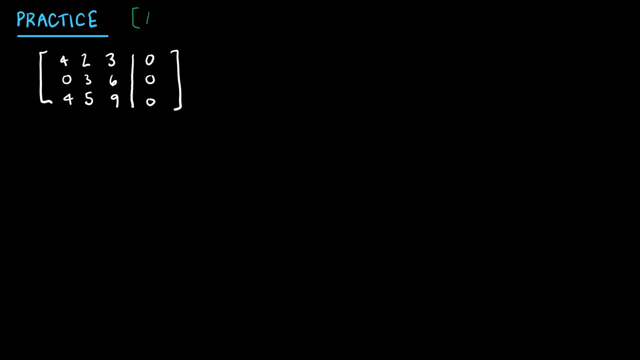 last equation, which is to turn this into reduced row echelon form and then write it as a parametric vector equation or parametric vector form. So, again, the first thing that I would do is I want these guys to be zeros, So I already have one zero exactly where I want it. 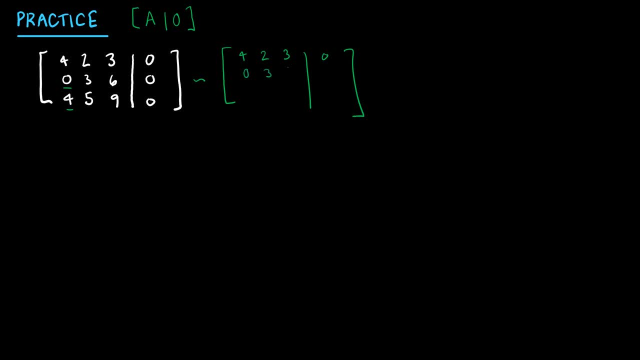 0, 3, 6, 0.. And then I would just take row 1 minus row 0, 3. So that gives me 0, negative 3, negative 6, zero. From here I can see I'm going to have a pivot here at 3.. 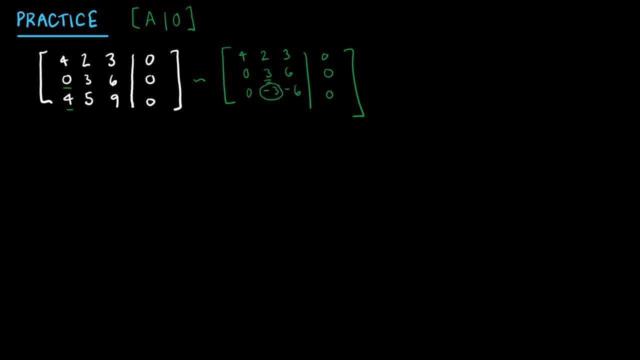 So that means I need this guy to be a zero. It looks like I can just add rows 2 & 3 together, which is going to give me row 1 exactly as I had it. I haven't touched row 1, and that's often the case. This guy is 0,, 3,, 6, zero. 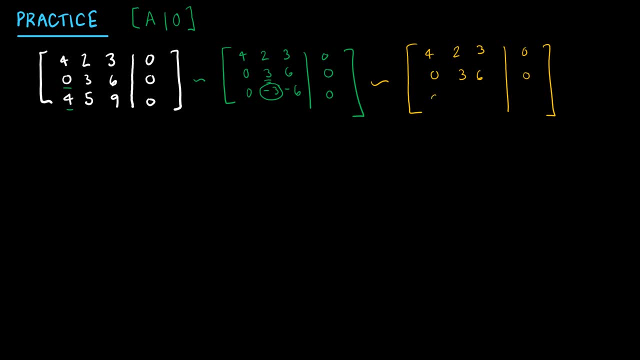 0, 3, 6, 0.. And then row 2 plus row 3 gives me 0, 0, 0, 0.. So again, I can see that x3 is free. Now, don't think x3 will always be the free variable. That's just what we ended up with. 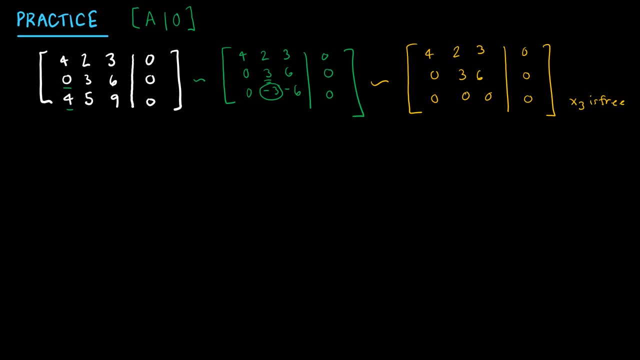 in this case and in our last example, From here I'm going to continue doing my row operations, So I'm going to end up with: let's turn this guy into a 1.. So 4,, 2,, 3,, 0.. Let's take everything in. 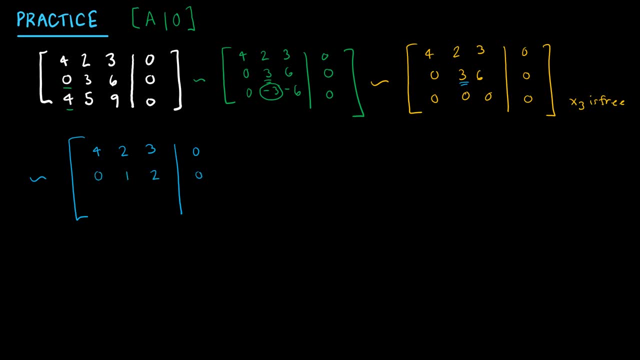 row 2 times a third And obviously row 3 is remaining exactly the same, And now I really want this guy to be a 1 if possible, But more than that, I really need this guy to be a 0.. So I'm going to continue, I'm going to take, I'm going to leave the 4 alone for now, I'm going. 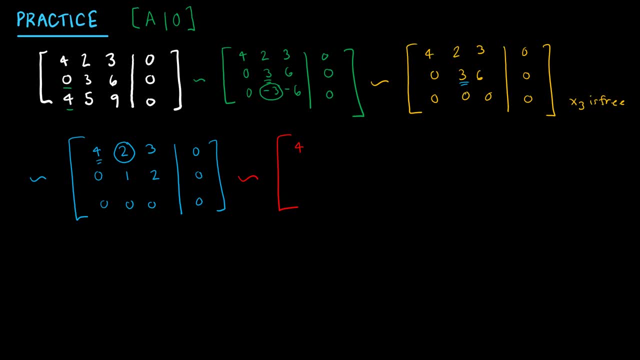 to take negative 2 times row 2.. So that's going to give me 0 here. So that's negative. 4 plus 3 is negative 1.. In this row: nothing changed. In this row: nothing changed. So I'm getting closer. 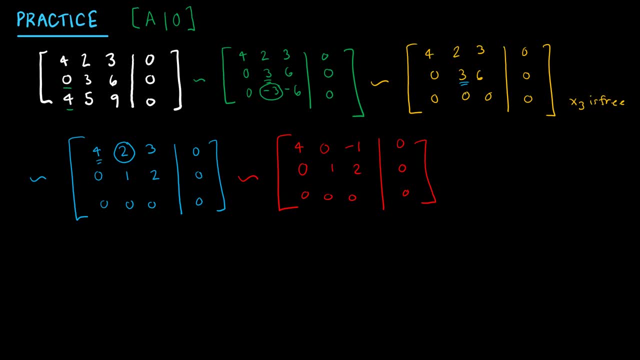 to where I want to be. And again, you don't have to in this step, but I'm going to. I want this guy to be a 1.. So I'm going to take negative 2 times row 2.. So I'm going to continue. So I'm. 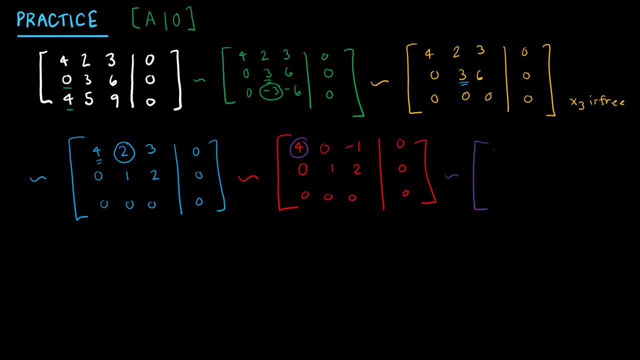 a one. so I'm going to take a fourth of everything. So that's going to give me one zero, negative one fourth. This guy is zero. one, two, zero and then zero, zero, zero, zero. So again the way that we did. 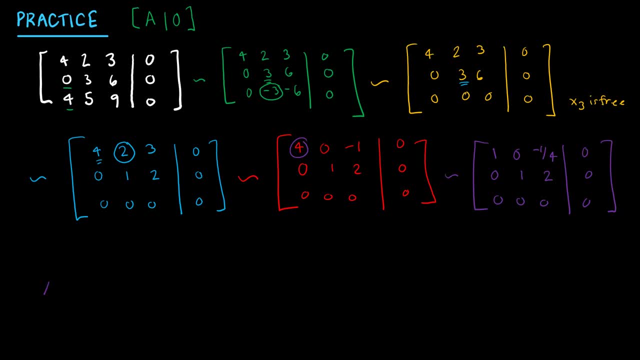 this before we wrote it. oops, I was going to change color there. We wrote it as just a set. I'm going to go ahead and write this as x one, x two x three. So what does that give me? Well, x one. 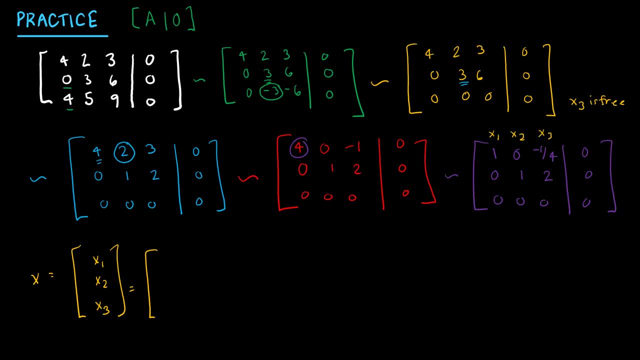 minus one fourth x three is equal to zero, So x one is equal to one. fourth x three. x two plus two x three is equal to zero, So x two is equal to negative. two x three And then x three is free, which means again, if I factor out x three, then I have one fourth. 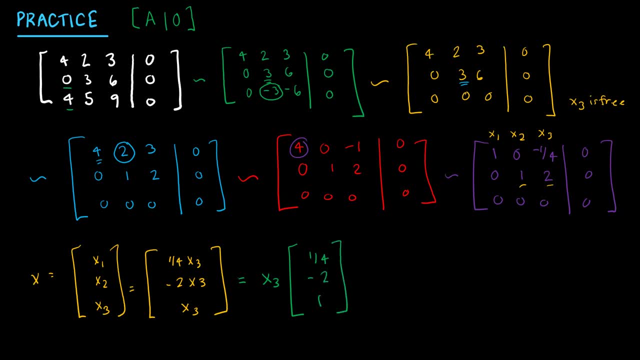 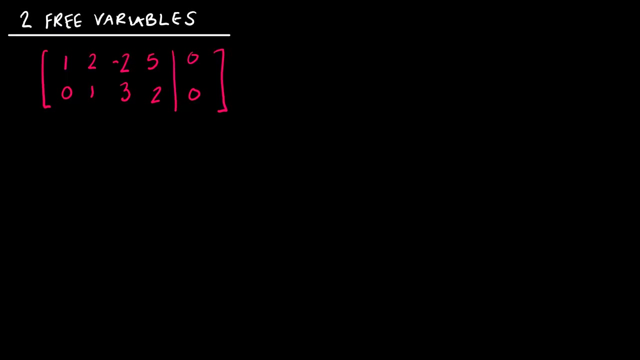 negative two one. So again, I'm able to then say that this is in fact in the correct parametric vector form, because I have some constant t times, some vector t V, And that's exactly what I want it. Let's do one more example here, And in this case I want to look at what happens when we have more. 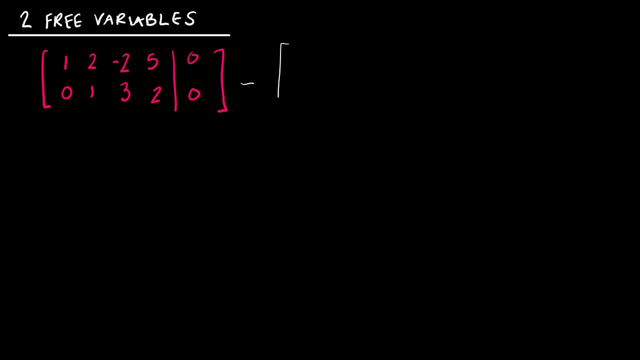 than one free variable. So again, it looks like I already have this one exactly where I want it And that's a pivot. And this guy is a pivot I already have. this guy is a zero. I need to turn this guy into a zero. So what I'm going to do is I'm just going to rewrite this one, So I don't. 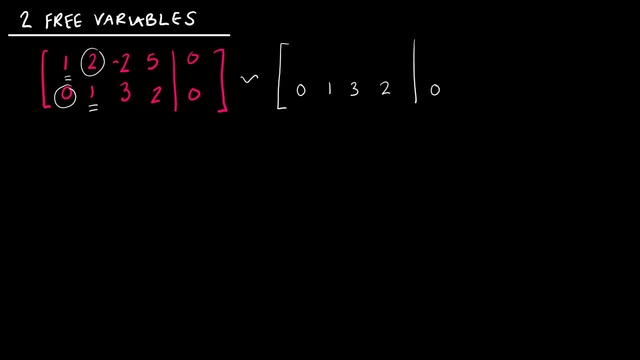 change a darn thing there. And row one: I want this two to be a zero, So I'm going to take negative two times row two plus row one. So negative. two times zero plus one is one negative. two times one plus two is zero negative. 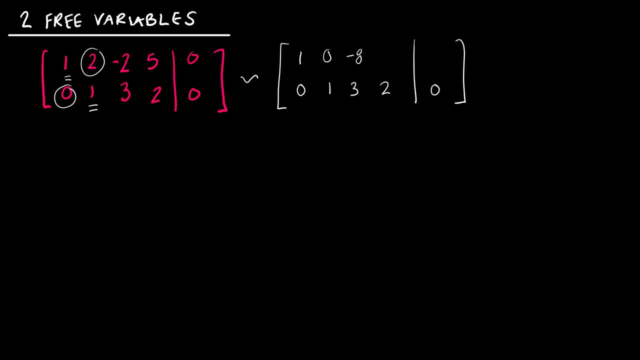 two times three plus negative two is negative. eight negative two times two plus five is one and, of course, zero. So what I have now is similar to what I had before and we can see that x one and x two are assigned and basic. 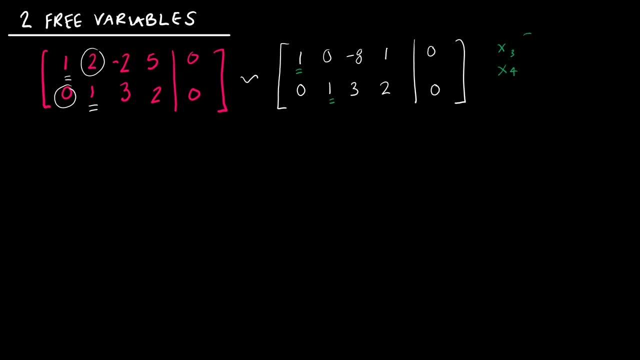 variables. essentially, x three and x four are both going to be free variables. So how am I going to write this? Well, I could say that x one minus eight, x three plus x four is equal to zero, and that x two plus three, x three plus. 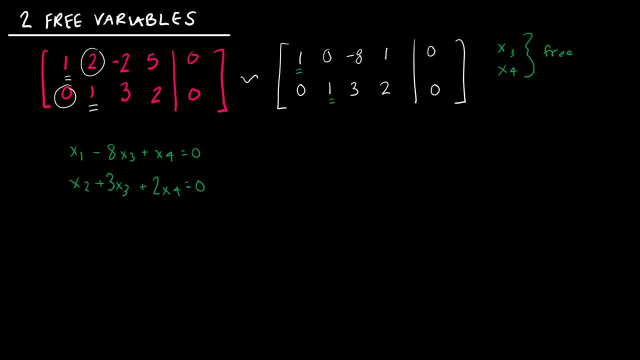 two x four are equal to zero or is equal to zero, And if I'm then writing my solution, x one would be eight x three minus x four. x two would be negative. three x three minus two x four. x three would be excstatisizcs three because it's free, and x four would be x four because it's free. 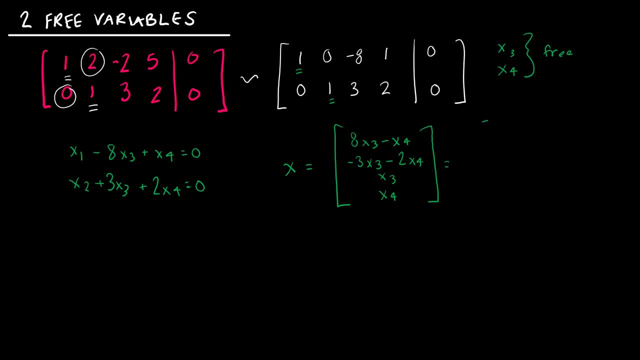 And so now I can write this a little bit differently. I can say: this is eight x three negative three x three x three and zero plus this guy is negative x four. this guy is negative two. award three x4, this guy is 0 because there's no x4, and this guy is just x4. So now what I can do is I can say: 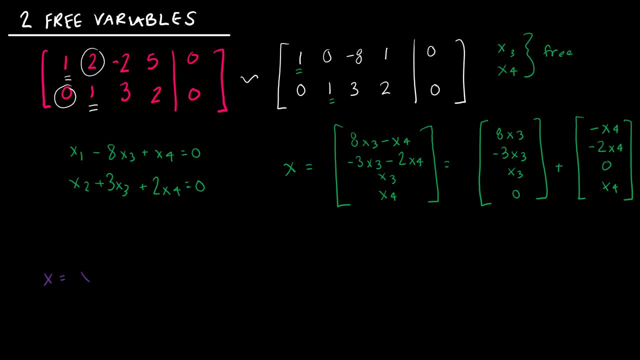 that x is equal to again factoring out that x3,, I end up with 8, negative 3, 1, 0.. And factoring out x4,, I get negative 1, negative 2, 0, 1.. And again is this written in parametric.